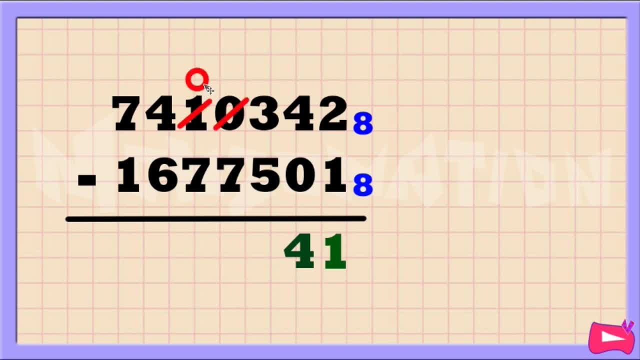 borrow from 1, so 1 becomes 0.. In the octal number system the base is 8, so the borrow is always 8.. So now let's put 8 here, Borrow. So we take borrow from 8, so 8 becomes 7.. Borrow 8.. The next step is to add 8 to. 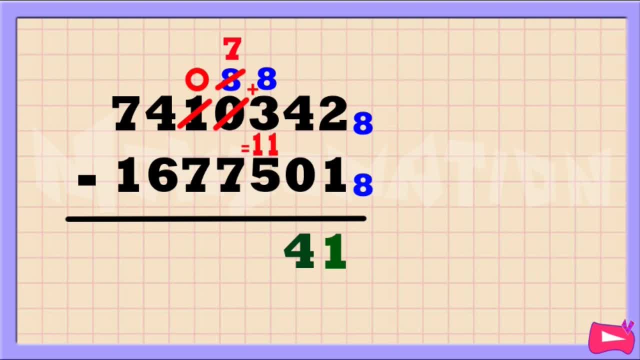 our minuend, which is 3.. 8 plus 3 is 11.. So 11 minus 5 is 6.. Next column: 7 minus 7 is 0. 0 minus 7.. We cannot subtract this because 0 is smaller than 7.. So we take borrow from. 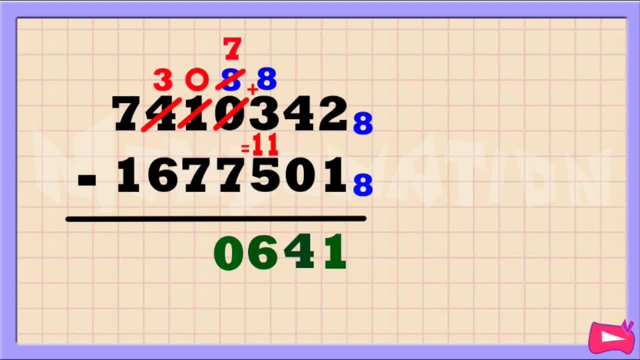 the next digit, which is 4.. So 4 becomes 3.. Borrow 8.. Next, 8 plus 0 is 8., And 8 minus 7 is 1. 3 minus 6.. We cannot subtract this because 3 is smaller. 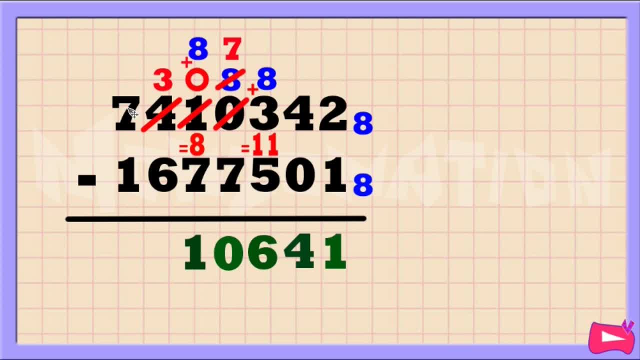 than 6.. Then we take borrow from the next digit, which is 7.. So 7 becomes 6.. Borrow 8.. Now let's add: 8 plus 3 is 11. And 11 minus 6 is 5.. And for the last column, 6 minus 1. 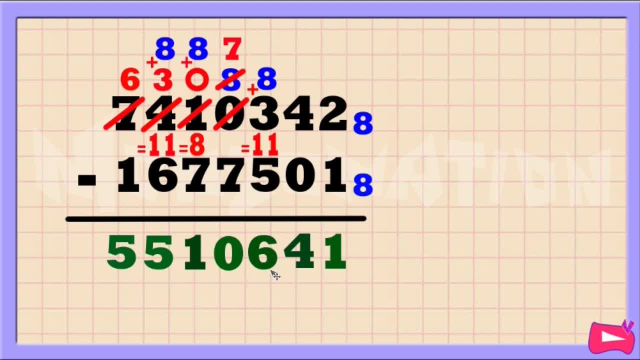 is 5. And the answer is 5510641.. We will write a little 8 down here to indicate that this is an octal number base: 8.. Now, if you'd like to check if your answer is correct, let's put powers of 8 on each octal numbers. 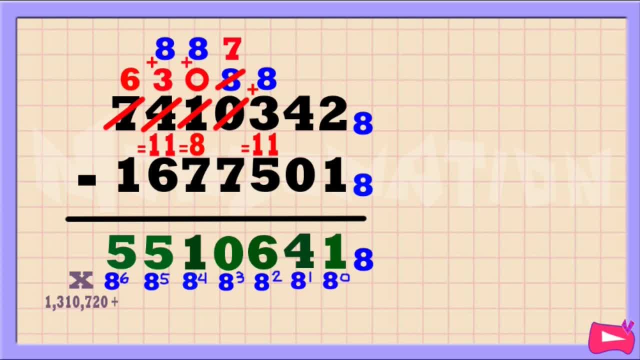 Then let's multiply it one by one: 5 times 8 to the power of 6 is 1310720.. 5 times 8 to the power of 5 is 163840.. And 1 times 8 to the power of 4 is 4096.. Then 0 times 8. 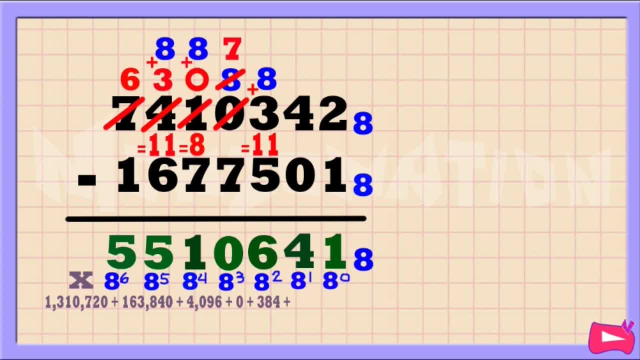 to the power of 3 is just 0.. Next, 6 times 8 to the power of 2 is 384.. And 4 times 8 to the power of 1 is 32.. Then, last octal number, 1 times 8 to the power of 0 is just 1..